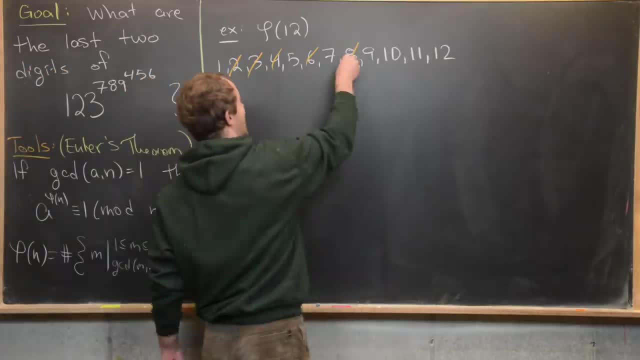 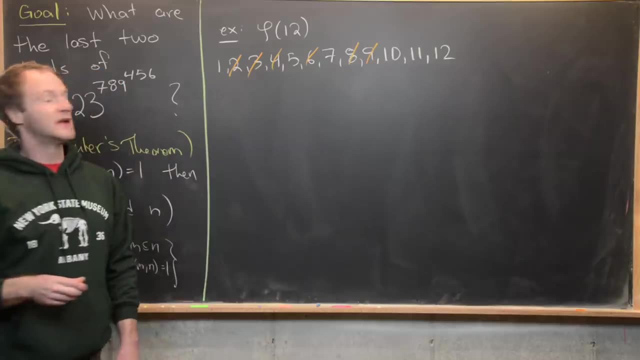 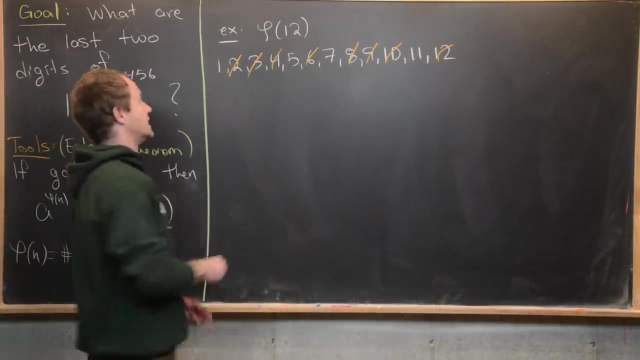 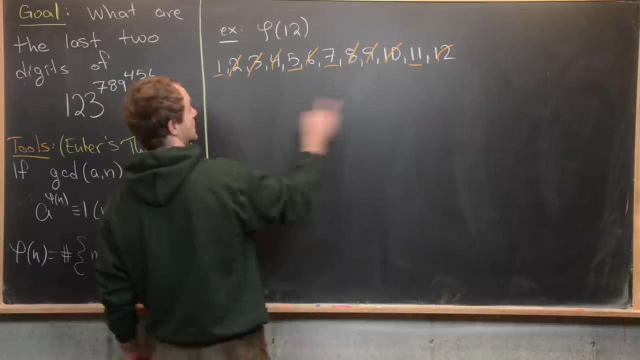 So they're automatically okay. Eight, So that is not relatively prime to 12.. Notice, their GCD is four. Nine, That's not relatively prime to 12.. Their GCD is three. So 10 and 12 are also not relatively prime to 12.. So in the end we have one, two, three, four numbers that are relatively prime to 12, that are less than or equal to 12. And so we have phi of 12 is equal to four. 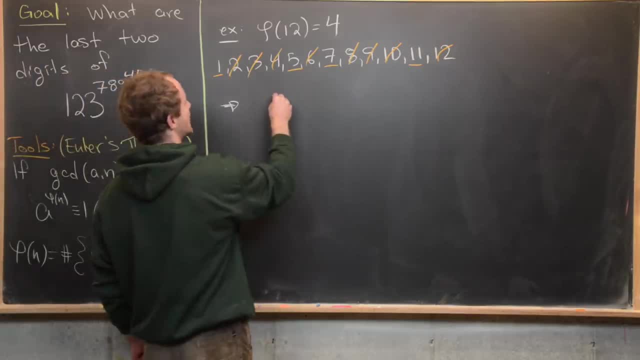 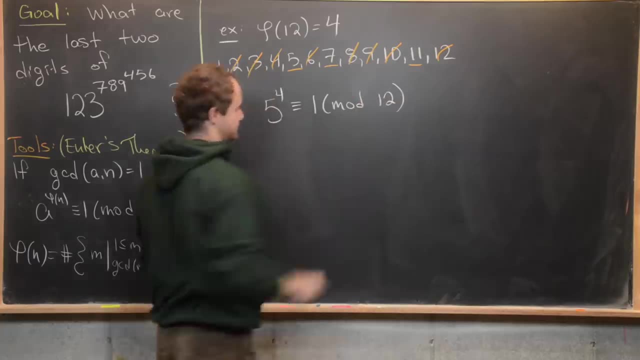 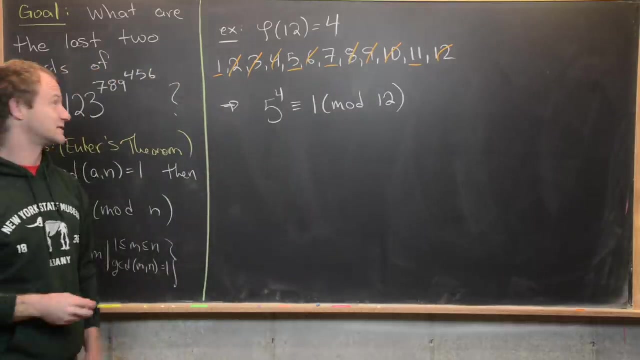 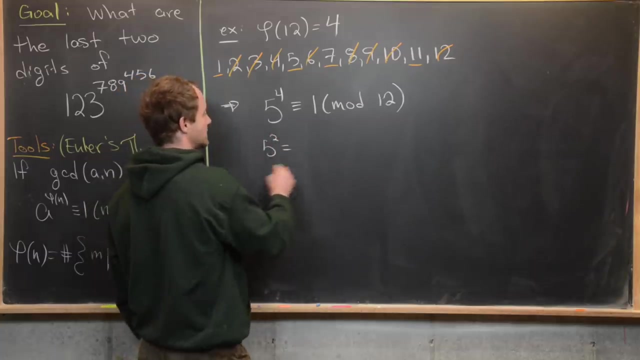 And now, applying Euler's theorem, we can see immediately that if we took five to the fourth power, that must be congruent to one mod 12.. And we can actually check this And in fact it. we don't always have to go up to this maximum number here. Sometimes we go up to a factor of that. So, for instance, if we take five squared, five squared is 25.. But 25 is congruent to one mod 12.. 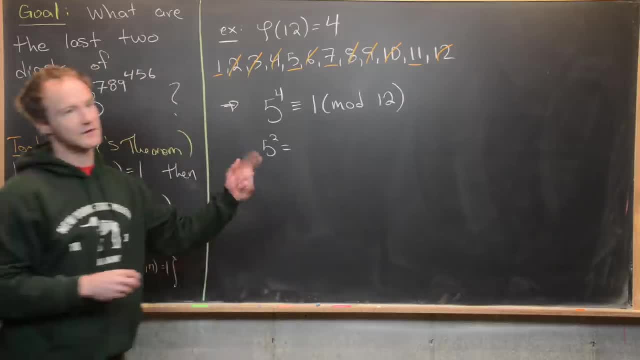 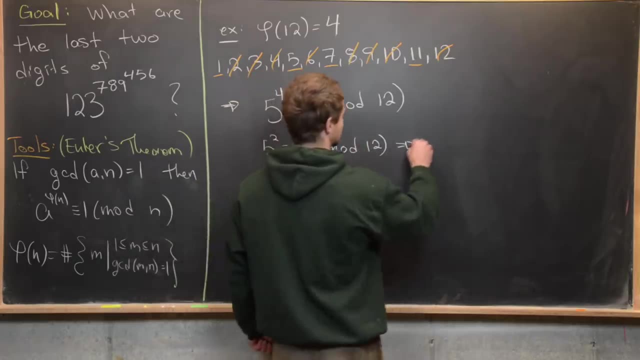 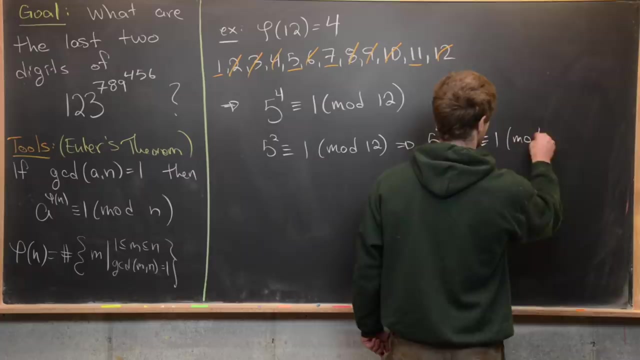 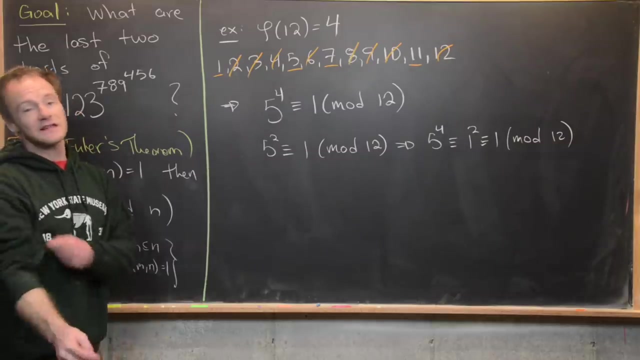 Because it's one more than 24.. So in other words, if you divide it by 12, you get a remainder of one. So here we have. this is one mod 12.. But that tells us that five to the fourth is going to be congruent to one squared, which is congruent to one mod 12.. So Euler's generalization of Fermat's little theorem checks out in this case. Now the next thing that I want to do is notice that we have a nice formula for Euler's generalization. 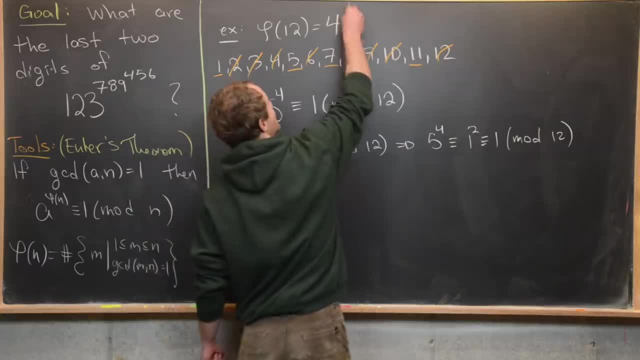 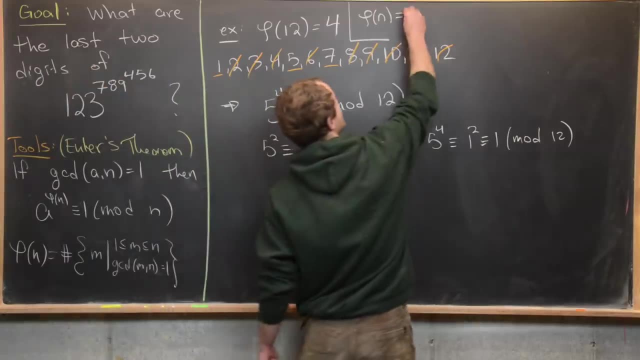 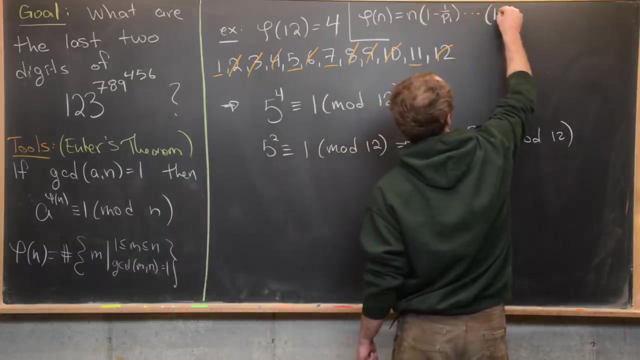 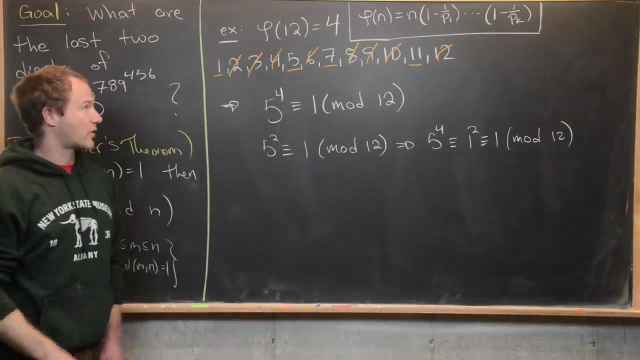 And we can just write it down. Maybe I'll fit it in right here. So phi of n has the following form: So it's going to be n times one minus one over p sub one, all the way up to one minus one over p sub k, where those pi's are all of the prime divisors of n. So via this formula we can calculate: 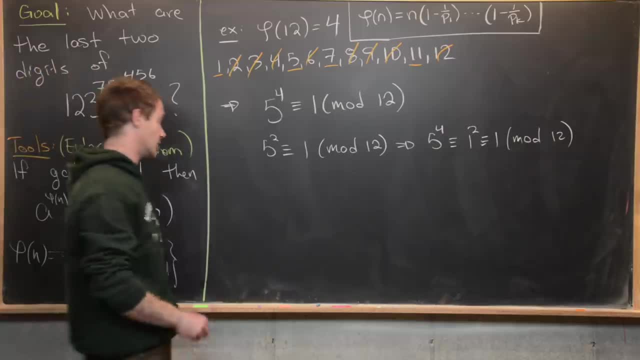 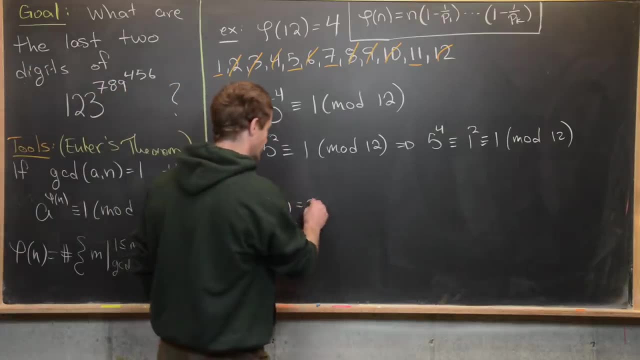 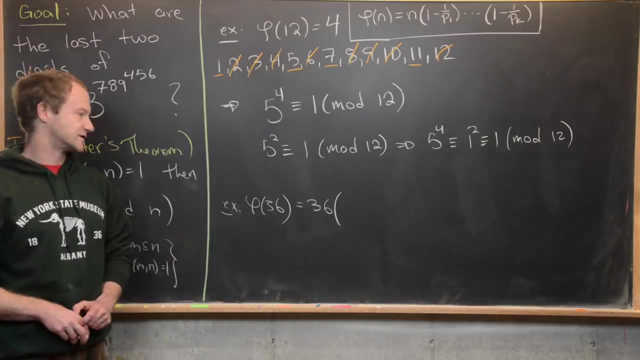 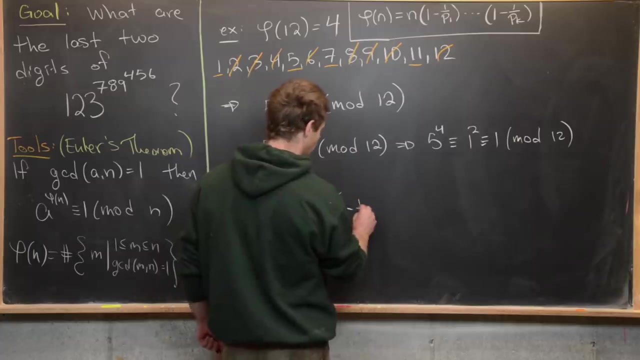 phi of a bunch of numbers very, very easily. So, for example, let's look at phi of 36.. So we know that's going to be equal to 36. And now we've got to multiply by one minus one over all of the prime divisors of 36.. So there are only two prime divisors of 36,, two and three. So we've got times one minus one over half, one minus one over third, like that. So that's all there is to it. 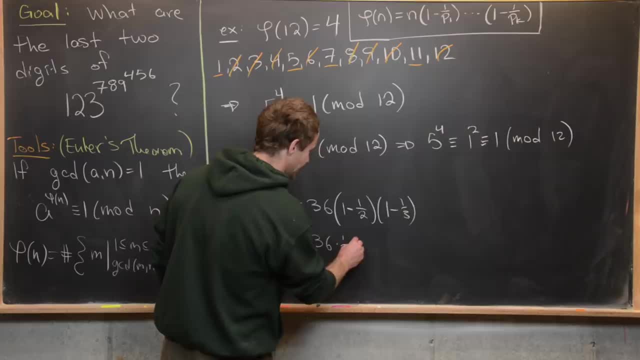 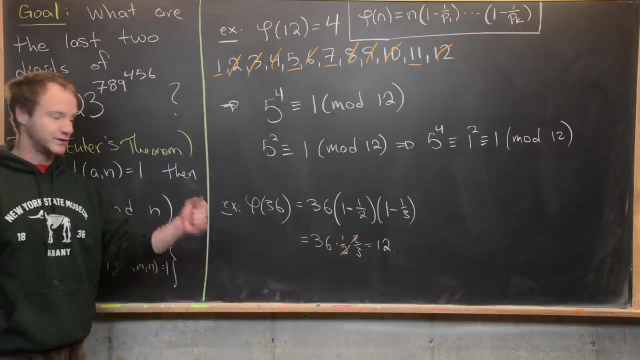 Notice that this is going to give us 36 times a half times two thirds. Notice we can do a little simplification there. Those twos cancel 36 over three is 12.. So that means phi of 36 is 12.. And I bet we could just write out all the numbers between one and 36, cross out the ones that are not relatively prime to 36, and we'd be left with 12 numbers once we were done with that process. 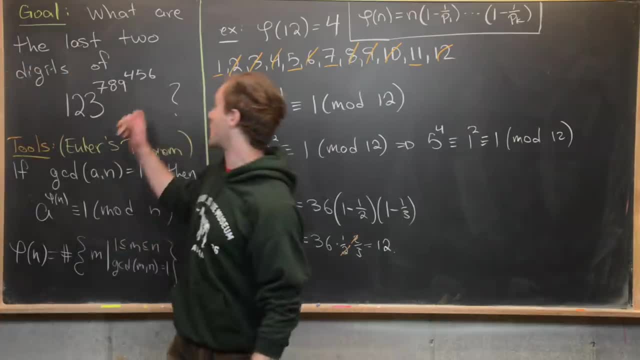 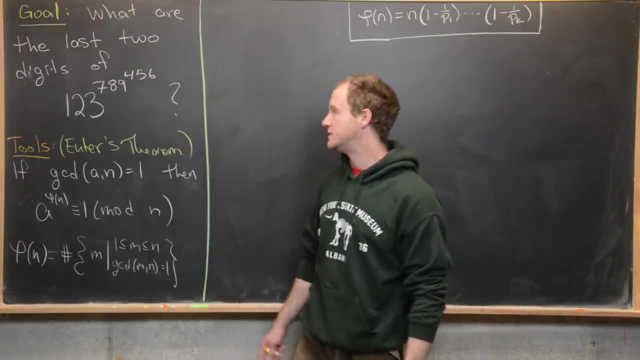 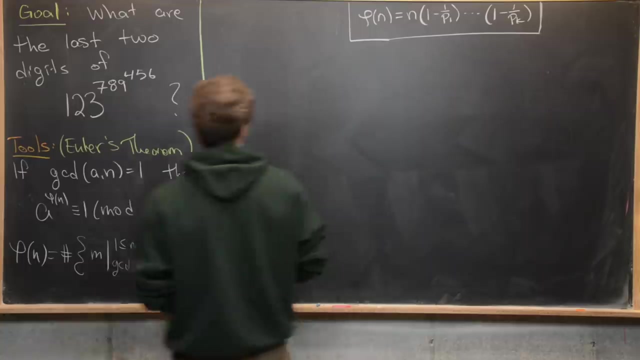 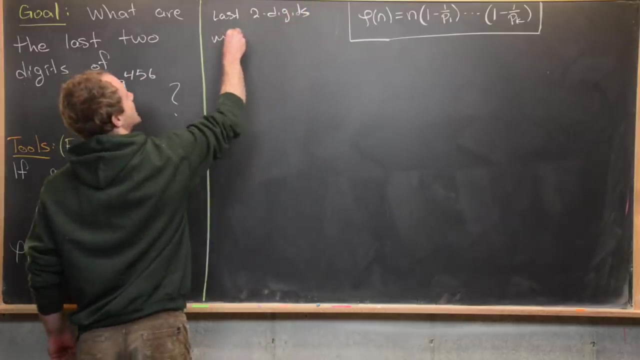 So now that we're kind of done with this, I'm going to clean up the board and we're going to launch into our main goal. Okay, now that we've done a little bit of review, we're ready to launch into our goal. So we're going to calculate the last two digits of 123 to the 789 to the 456.. And the first thing that I want to notice is, if we want to find the last two digits of anything, then all we care about is the reduction mod 100.. So notice the last two digits of anything. 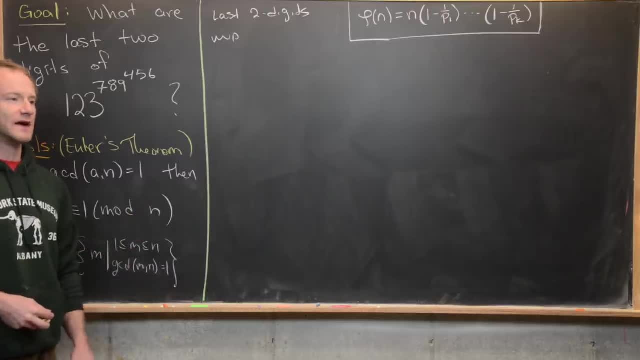 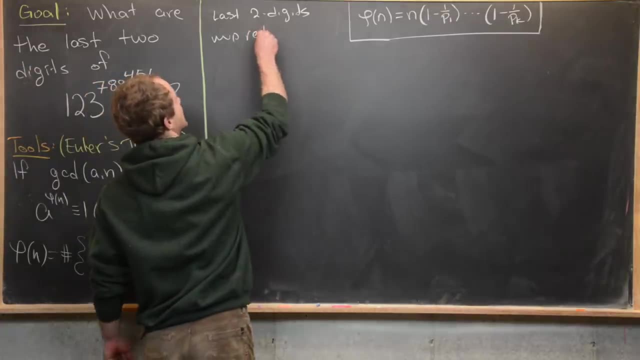 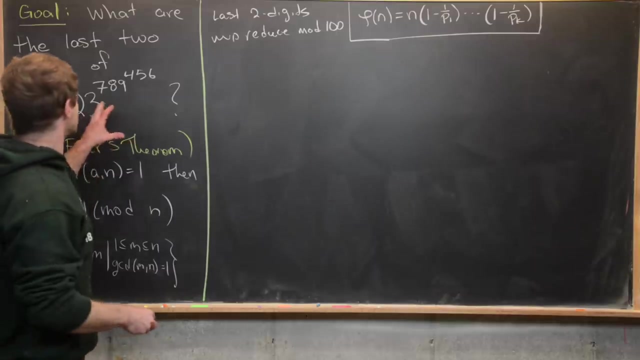 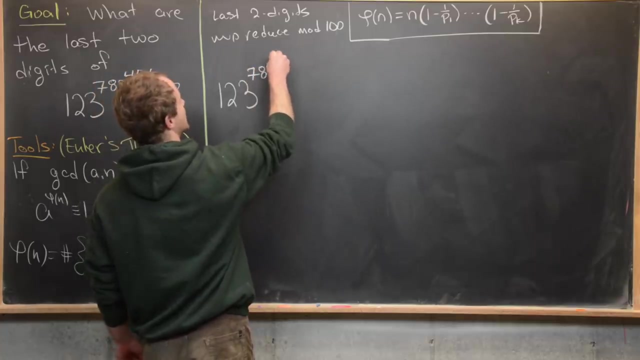 any number will be the remainder after dividing by 100. In other words, if we reduce mod 100, then all we're left with is what we want. So let's go ahead and put here: So we'll reduce mod 100. Great. But now let's go ahead and look at our number here. So we have 123 to the 789 to the 456.. Okay, so this whole thing needs to be. 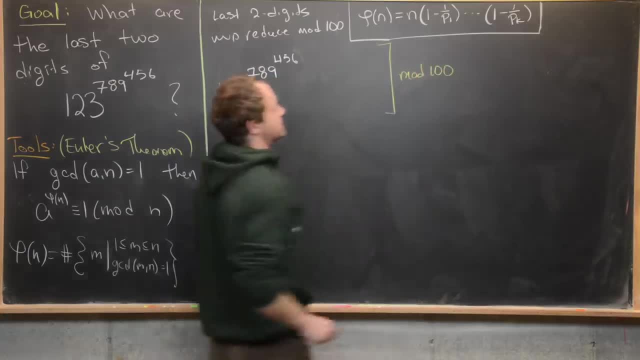 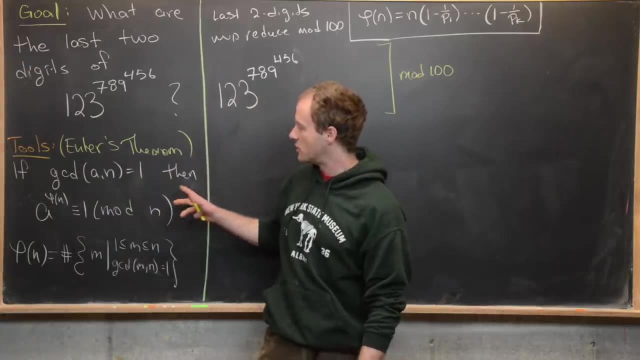 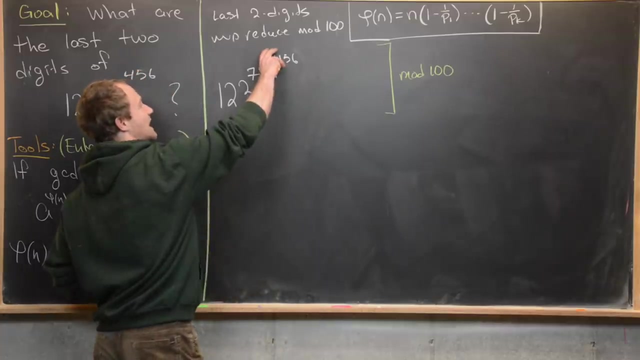 reduced mod 100. So that may seem still like a tall order, But we can look at Euler's generalization to Fermat's little theorem and notice that the exponent is operating mod phi of n. So notice, if we like, divide this exponent by phi of n and then keep the remainder. the remainder is the only thing. 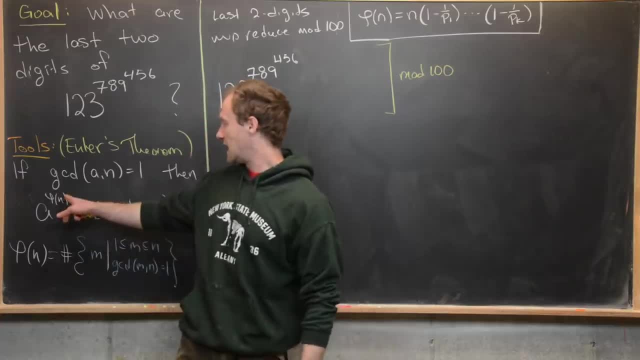 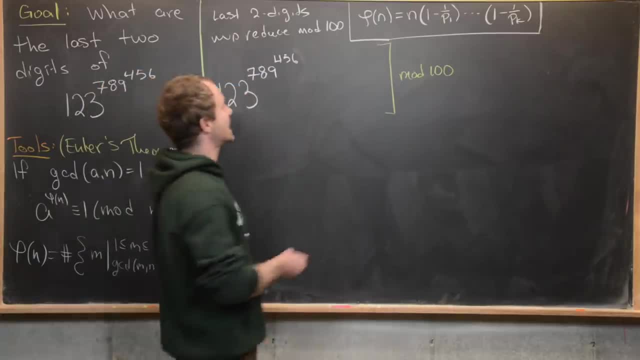 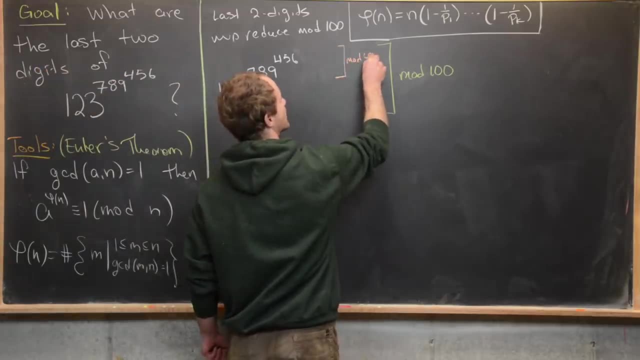 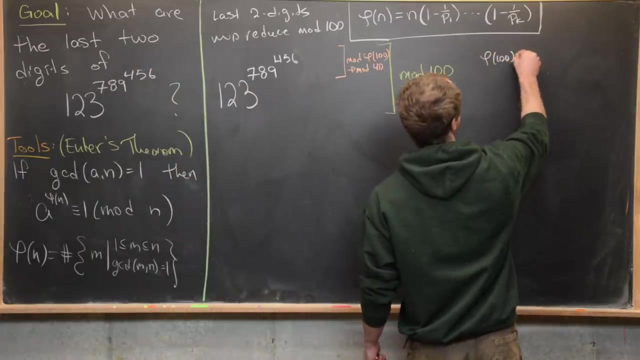 123 down to one, And so the takeaway here is that this exponent is happening mod the Euler phi function of 100.. Good, But I might as well point out that the Euler phi function of 100 is 40.. You know, maybe we can calculate that over here on the side. So, phi of 100.. So that's. 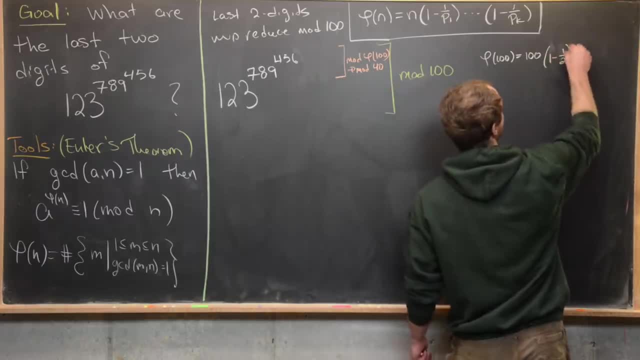 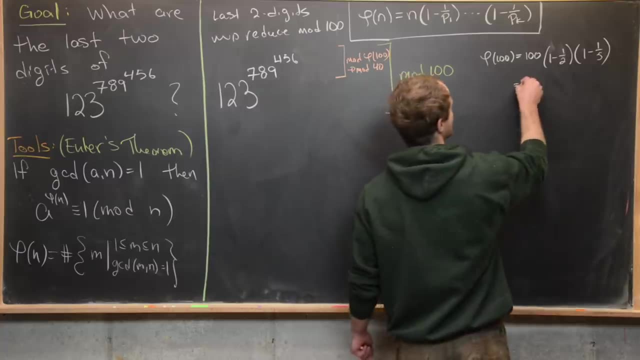 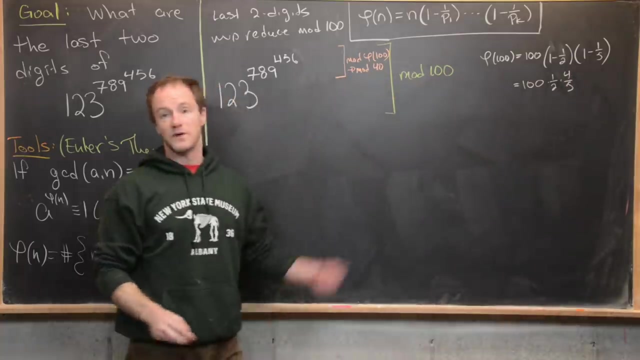 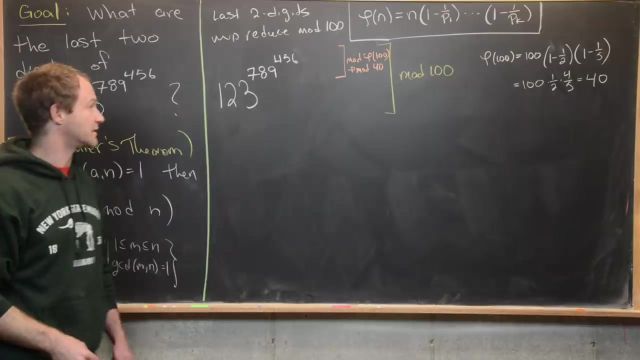 going to be one minus half times one minus a fifth. Two and five are the only prime factors of 100.. So let's see what that gives us. That gives us 100 times a half times four fifths, But then that very, very quickly becomes 40. So notice, we have 100 divided by 10 times four, So that's going to be 40.. Okay, But now we've got one more level of exponents here. 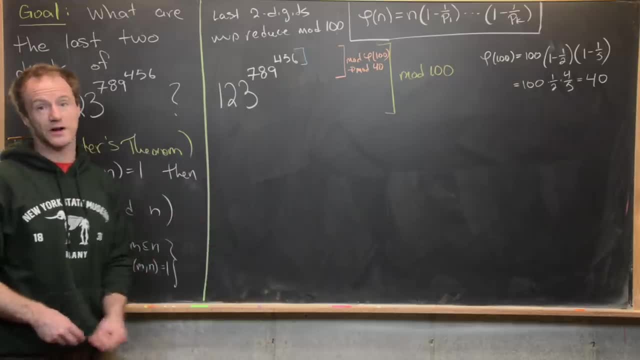 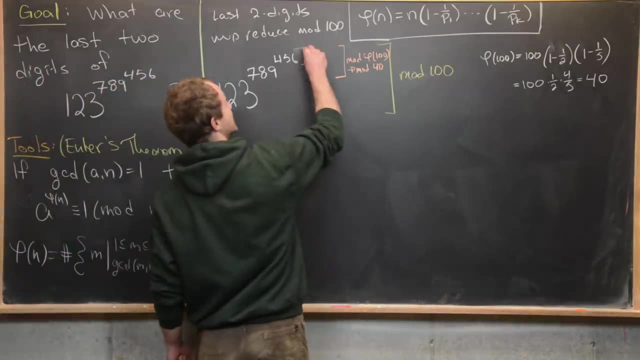 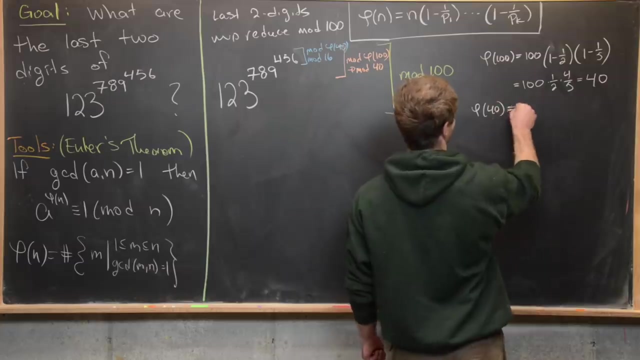 And this exponent will be working- mod phi of 40- just because we've got this Euler's theorem inside Euler's theorem, essentially. So, like I said, this is going to happen: mod phi of 40. And I'll just say that that's going to be 16. So this exponent is working: mod 16. Let's maybe go ahead and check that out over here. So we've got phi of 40. So what are the prime factors of 40?? They're also just two and five. 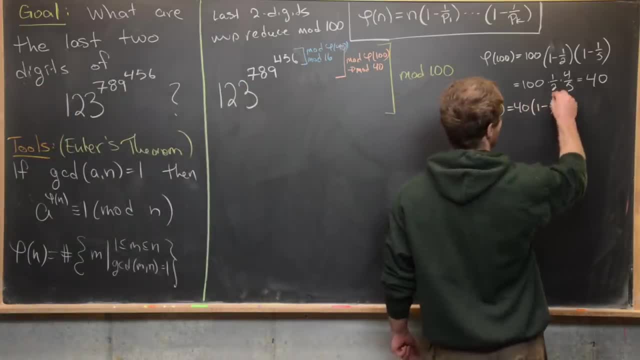 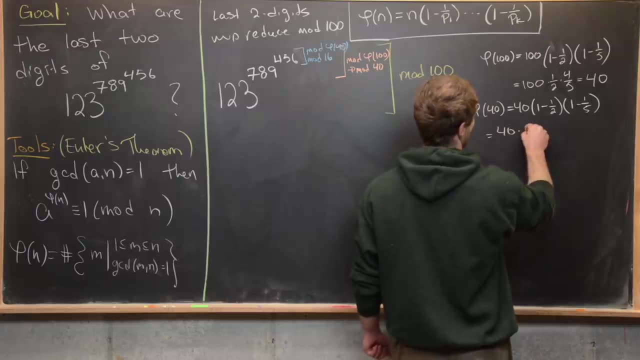 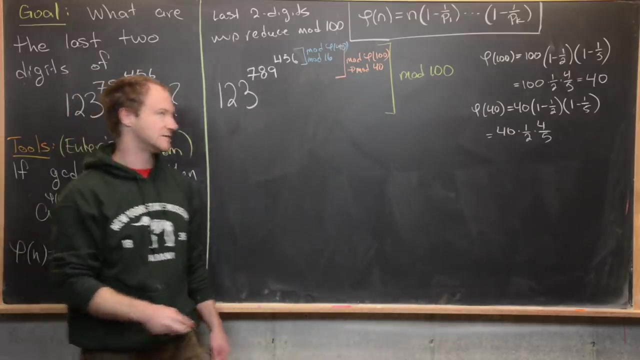 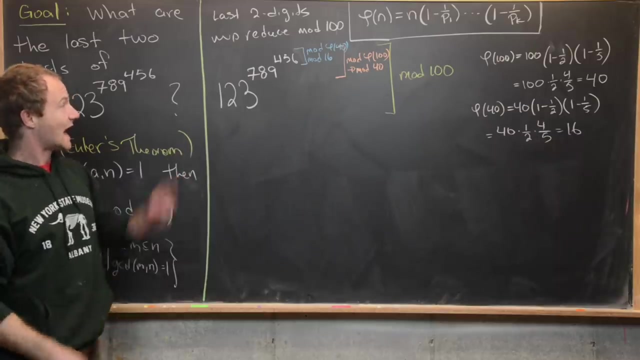 So we've got 40 times one minus half times one minus a fifth. So again, that's 40 times half times four over five. But notice, we've got 40 over 10 is four times four is 16.. So that's right. this is working mod 16.. Now we want to do some like division problems with remainder in order to reduce 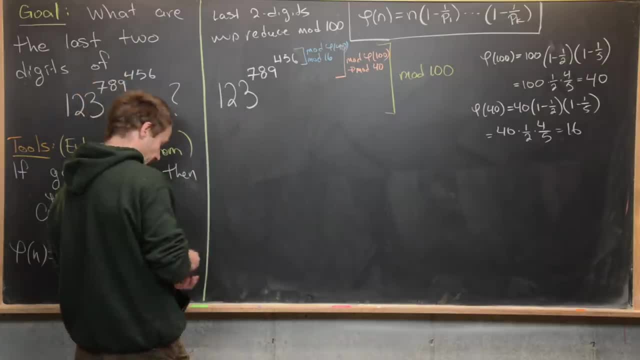 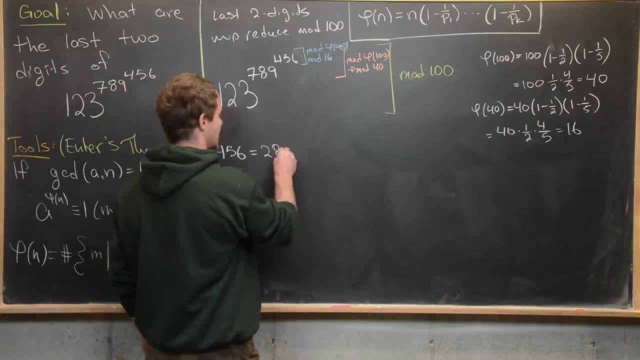 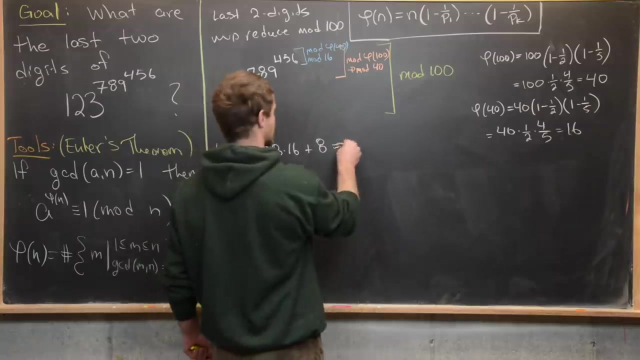 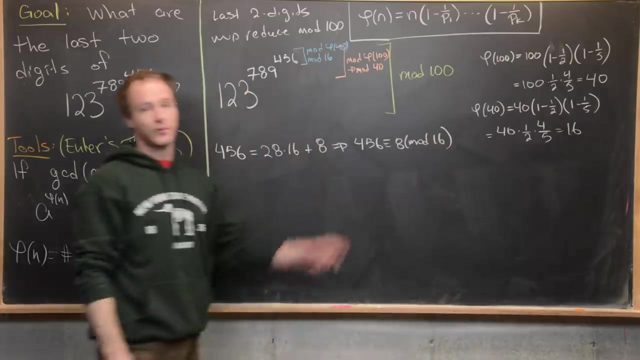 from the inside out. So notice that we have: 456 is equal to the following: So that's equal to 28 times 16 plus eight. So that's just easy division with remainder. So what that tells us is that 456 is congruent to eight, mod 16, which is a really important fact because again, this exponent in the exponent is working mod 16.. So we need to 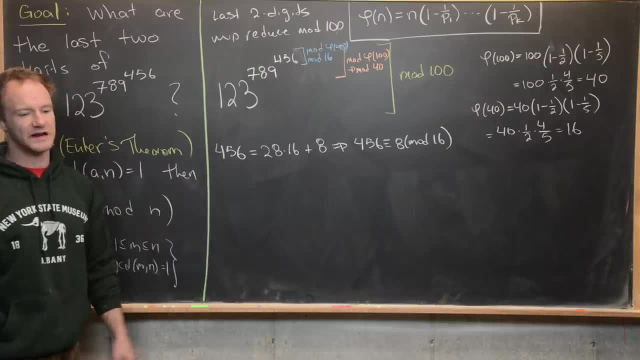 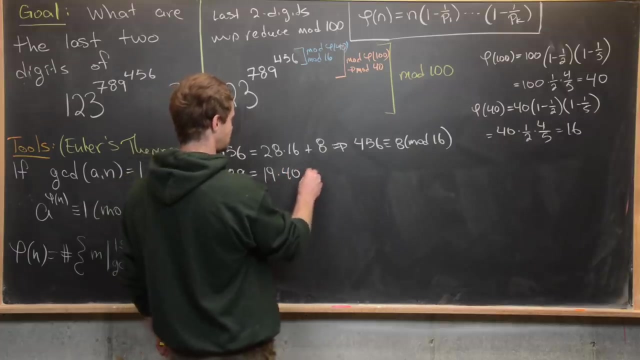 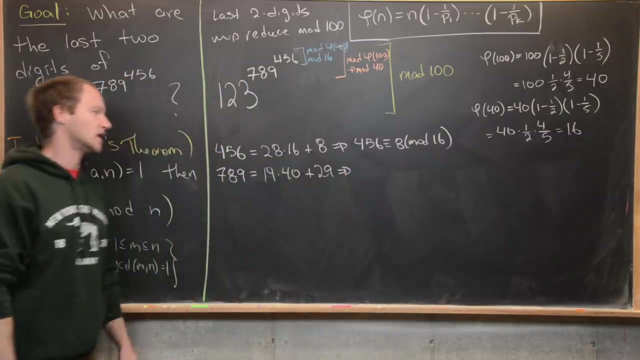 replace this 456 with eight, which is what we'll do in the next step. Okay, and next let's look at this: 789.. And we're going to look at that after dividing by 40, because we're reducing that mod 40. So that's 19 times 40 plus 29. So that means that 789 is congruent to 29 mod 40. So let's write that down. So 789 is congruent to 29 mod 40.. So 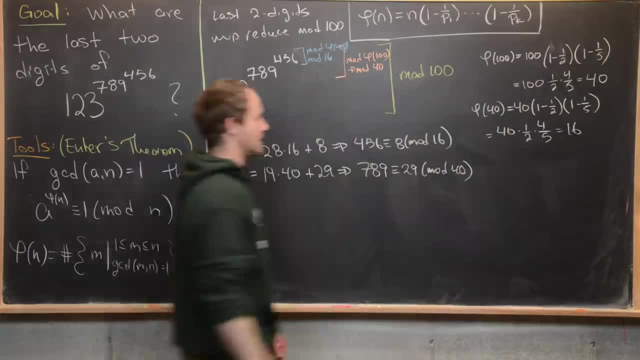 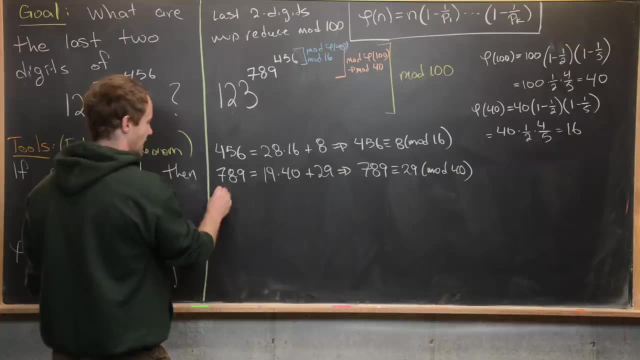 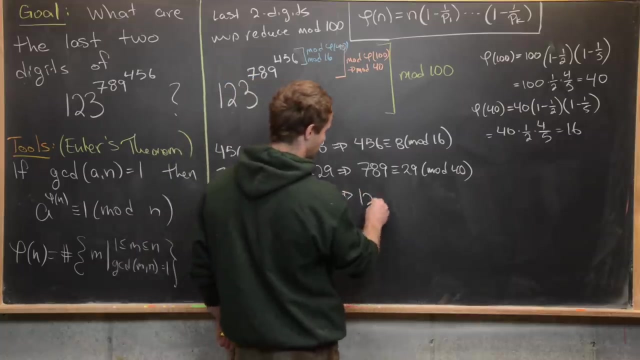 29 mod 40. great. now we've got to look at the base, and the base is working mod 100. so that means 123. well, that's easy to see. that's just 100 times 1 plus 23, but that tells us that 123 is congruent to 23 mod 100. good, now we want to put all of this together. 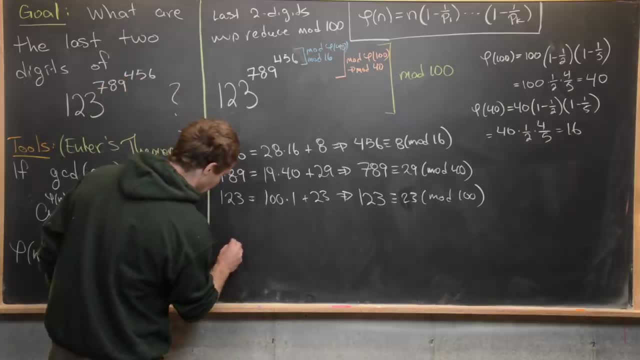 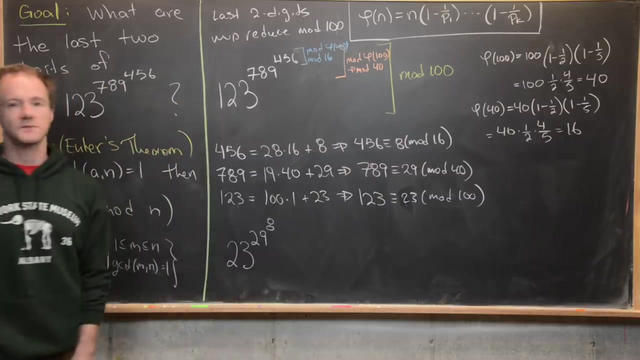 so we can reduce this one bit at a time. so this is going to be 23, and now we've got 789 goes to 29, to the 29, and then we've got 456 becomes 8. okay, good, but that might seem still a little bit tricky. 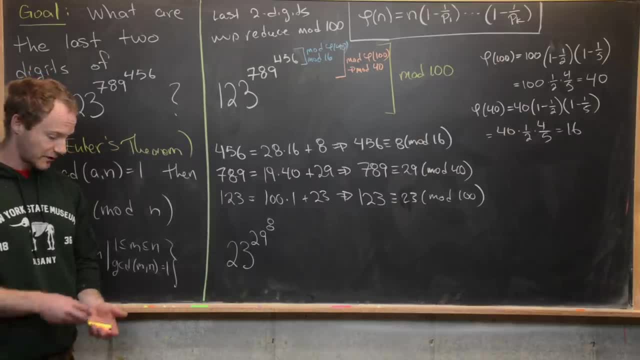 like, maybe this is too much calculation, more than we want to do, but we can use a simplification rule here and we can use a simplification rule here, and we can use a simplification rule here and here, and that is working with negative numbers instead of working with positive numbers. 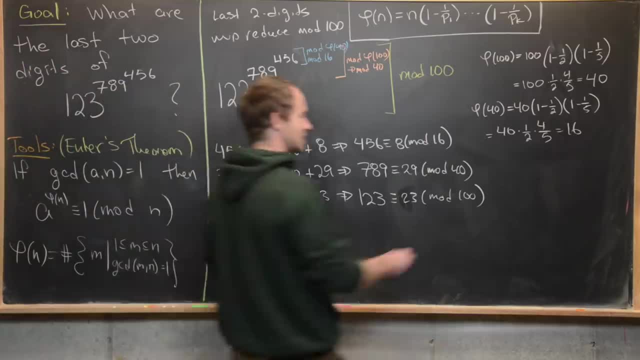 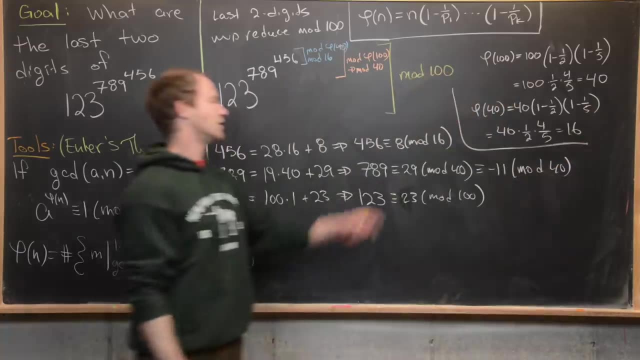 so notice, if we have 29 mod 40, that's going to be congruent to minus 11 mod 40. and how do we see that so quickly? well notice, if we do, uh, 29 minus 40, we're going to get minus 11. so we've got.